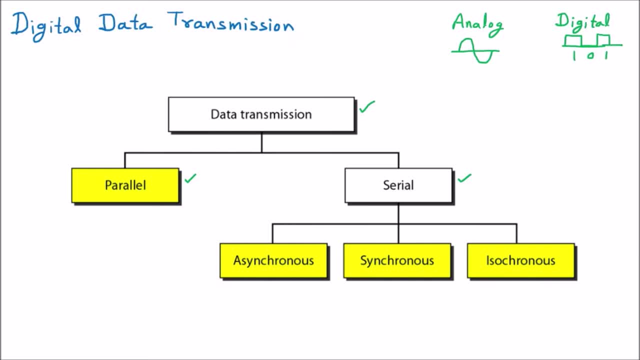 type of data transmission: One is parallel and second one is the serial. Now I am taking one example to make you understand. Let us suppose that we are having the sender this side and from there we are having the multiple lines. Let us suppose that these are the multiple lines which? 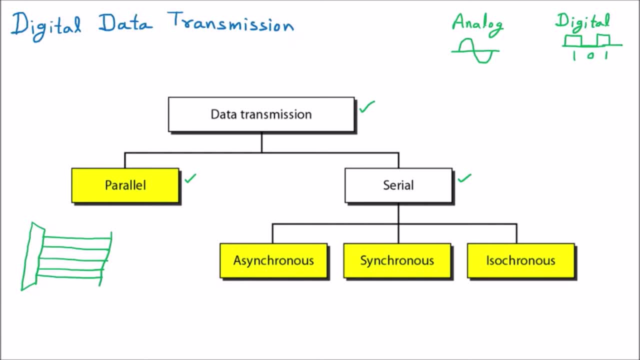 are going from one sender to other receiver. So now you can see that there are multiple lines which are going. So this is the example of parallel communication If I say that 1,, 2,, 3,, 4 and 5.. 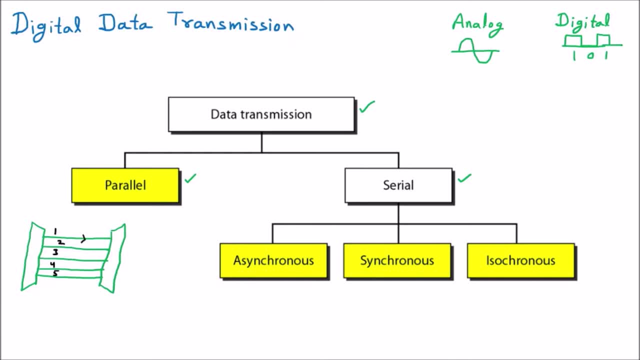 So these are the five lines which are sending the data. So data is moving directly from these lines. Now assume that one line can send one bit of data. How much data I can send at the same time? So five bits can be sent at the same time. 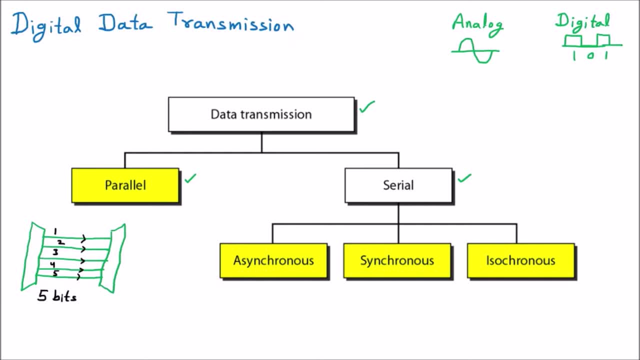 So this is called the parallel transmission. Parallel transmission means there are parallel lines. If I have to send the five bits, then I need five lines. If I have to send the 15 bits, then I need the fifteen lines First. I'm taking an example. let us suppose that one line is sending the one bit. 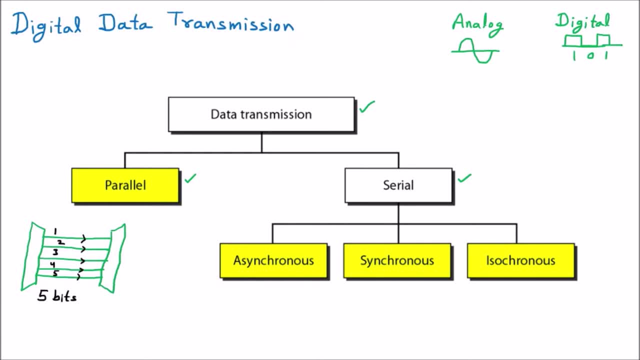 Talk about multiple lines. So you can see here that one line is sending the one bit, Talking actually about next one we are having is the serial transmission. the serial transmission we are learning from very first day. let us suppose that there is a sender this way and there is a receiver. 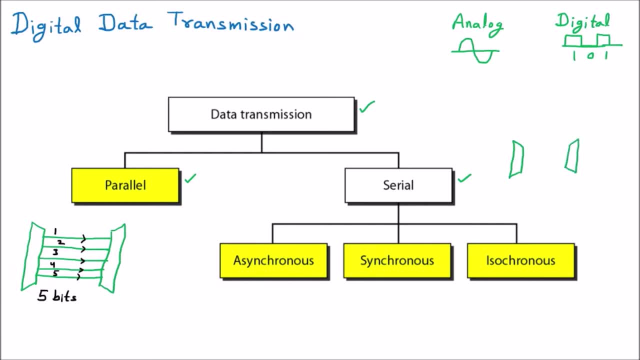 at this side. now, here we are sending through one wire, one line, so it is a single line on which we are sending the data. so that is called the serial transmission. let us suppose that at the same time we are having the five bits of data. but it will go bit by bit. only one bit can go. so there we can. 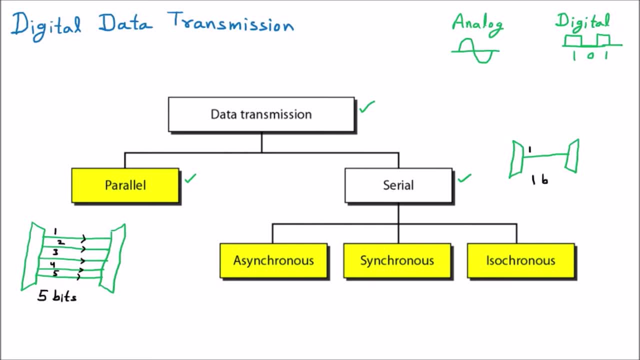 say that only one bit can transmit at a time. so this is the serial transmission. so these are the major categories of the data transmission in the digital form. one is parallel and second one is the serial. so now we are discussing the parallel transmission and afterward we will see the 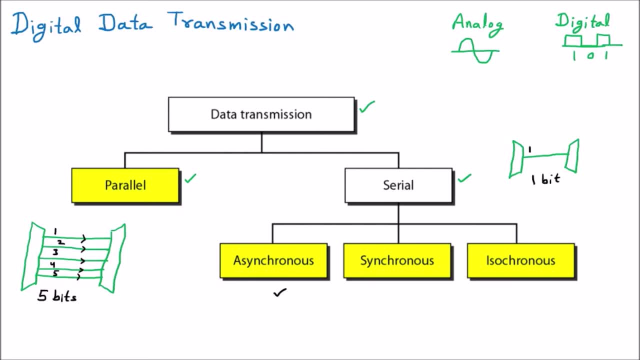 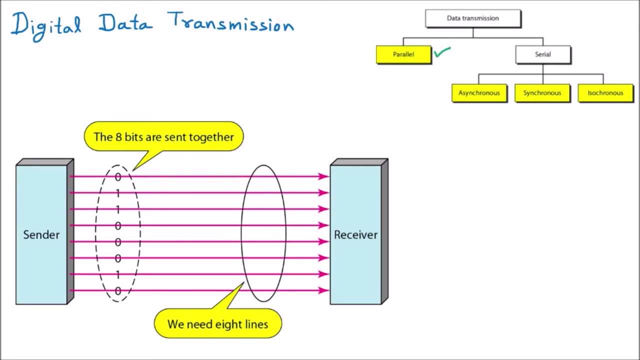 further categories of the serial transmission. so we are discussing the serial transmission also which is asynchronous, synchronous and isochronous. so this whole diagram we will discuss one by one. but first of all we are going to the parallel transmission. so now we are discussing the first category, which is the parallel transmission. so we are writing here it is: 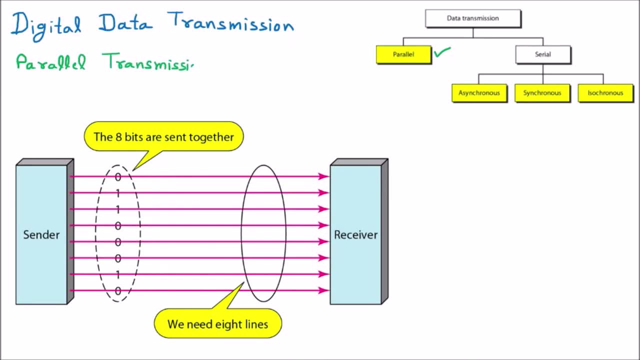 parallel transmission. so, guys, now this diagram is very much clear to all of you that this is our binary transmission are fine, so all these points are written down here, but is that? they are not shrinking our video? and we are calling it data transmission. so lets take it again. so let us. 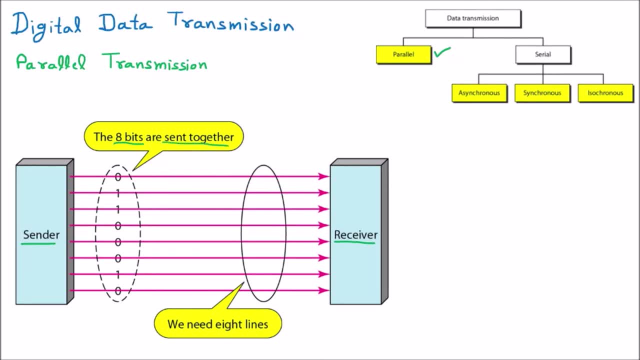 look at the clear stuff, okay. so let's look at the clear плюс case for this data transmission here. first of all, let us look at the map for this data transmission. so if you are looking here, let us look at this data transmission chart. work with the words following the first. 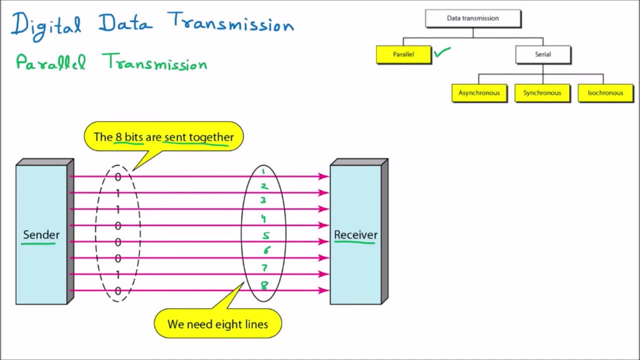 item of the data transmission. that is the present element from the previous screen. so let us look at parallel transmission and that was about 3 ICU stands and I am going to look at these patterns. the 8 bits bits can be 0 and 1 because we are learning the digital data transmission. then for 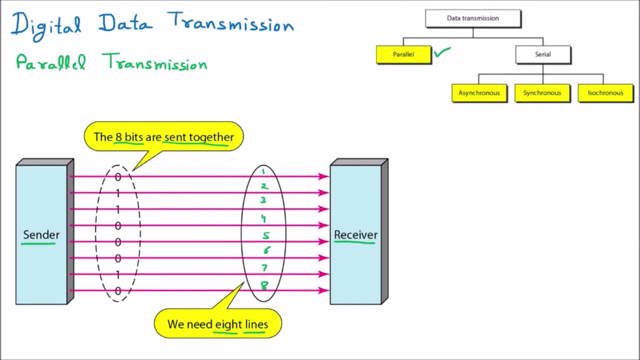 sure we are sending the digital signals. so if i talk about the definition, then we can say that we can send, or we can say the multiple bits are sent with each clock tick. well, that is very interesting. each clock tick means whenever we are saying a second, whenever 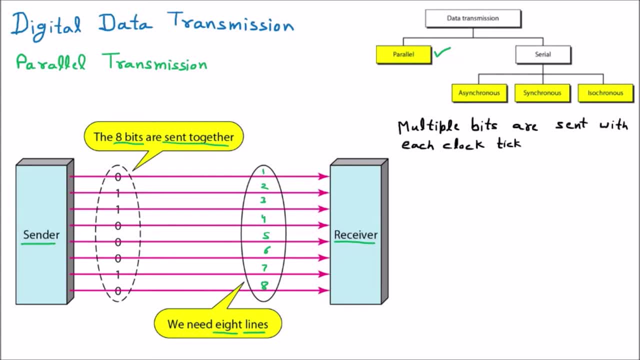 the clock move, a second moves right. a clock tick- we say it as the clock tick. so at a second moved, the multiple bits are transferred. so in the case of this diagram, whenever our clock tick moves, the 8 bits are transferred because there are 8 lines. so there is one more conclusion we can draw. 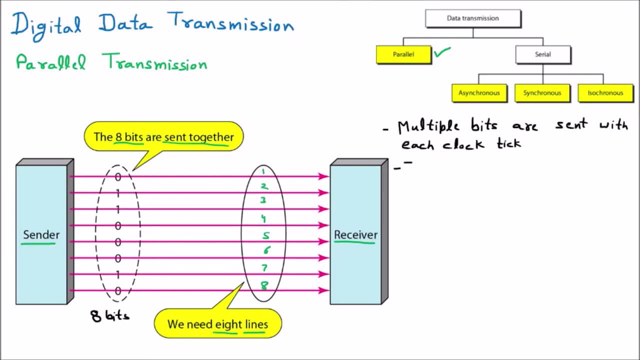 so that to transfer 8 bits there are 8 separate lines are required, means to send the 8 bits, we need the 8 lines, or to send the 20 bits, we need the 20 lines. so that is the important thing about the parallel communication. now we are moving towards the advantages. so if i say the advantages, 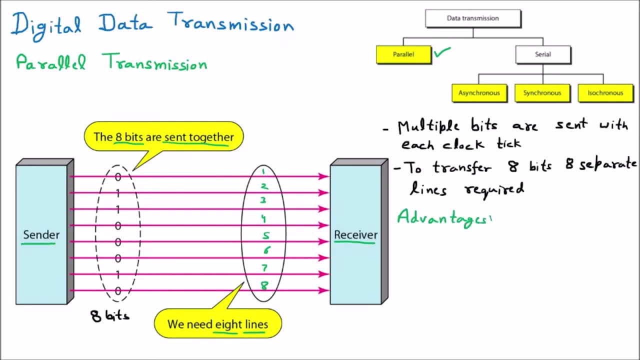 for the efficient Subsiddiary Transication, then the very first advantage of the parallel communication is high speed, so we can say that the speed is very high. the reason is there if you are transferring a data and you are having multiple lines to transfer and all. 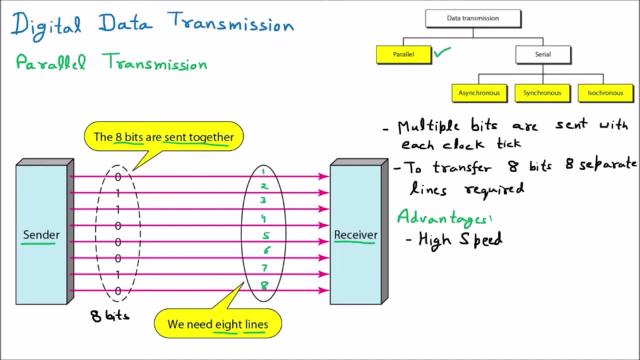 are in your control so obviously the speed will be very high. so that is the main advantage of the parallel communication. but there are various disadvantages also. so if i talk about thedisadvantage capabilities for session, So if I talk about the disadvantage, then the first disadvantage is the cost. We know that if 8 lines are there, then obviously 8 times the cost. Let us assume that I can send the data from one line, but I am using the 8 lines now. 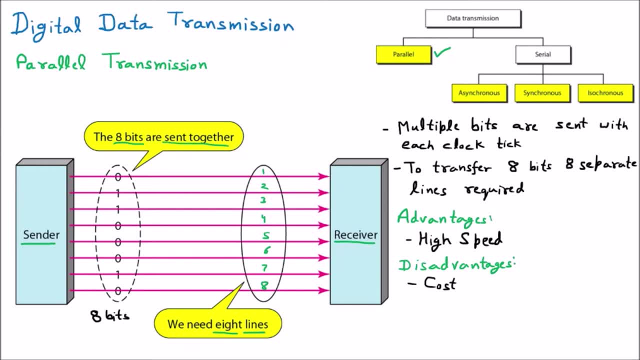 So 8 times more cost will be there. So cost is very high and also it is limited to short distance. So that is a major disadvantage. Let us suppose that you are having the 8 lines for sending 8 bits, but maybe you can send in your area or maybe you can send in 10 km, 20 km, but you cannot just send these 8 lines to complete city. 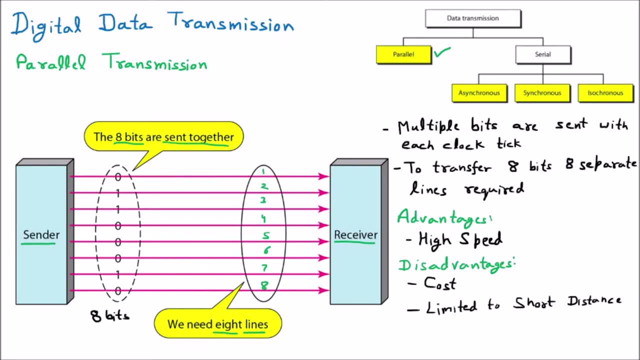 For your communication you are using 8 lines. That will be very, very costly, So long distance is not possible. So that is why we see that parallel is obviously better in terms of speed, but in terms of cost parallel is the worst. So that is why we are having the next type of the data transmission and that is called the serial transmission. So now we are learning the serial transmission. 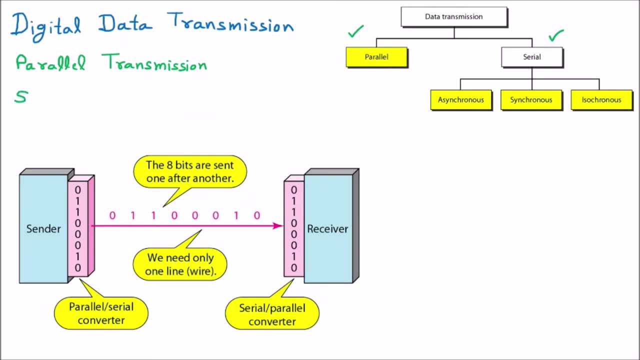 So I am writing here: This is the next transmission, which is serial transmission. So, talking about the serial transmission, we are having only one line, So you can see that only one wire is there, So this is only one wire through which we are sending the data. 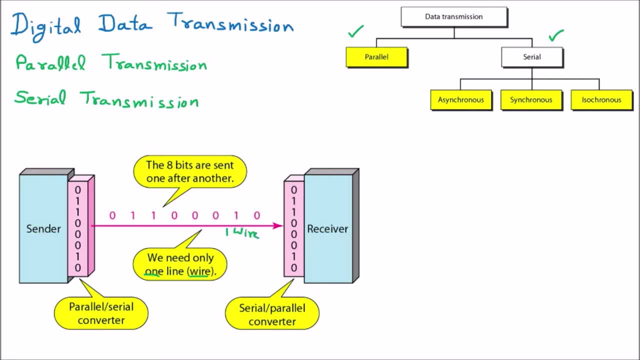 So I am writing here one wire or one line. Now if I have to send the same 8 bits, Let us suppose that these are the 8 bits Which I have to send. So these 8 will send one after another means they will go into the sequence: one by one they are sending. 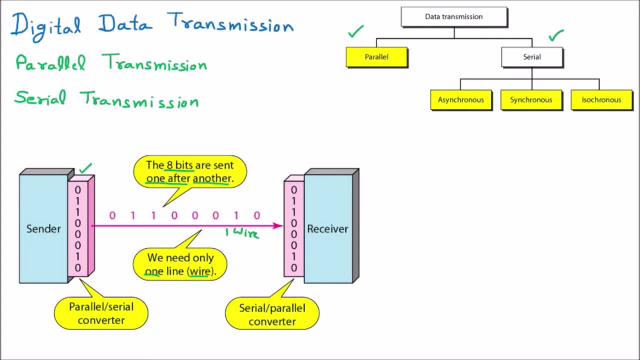 We cannot send them at the same time. So what will be the speed? speed will be only 1 bit. That means only one bit will be sent. If I assume that in the previous example, in the parallel communications, the speech mode, Let us suppose that 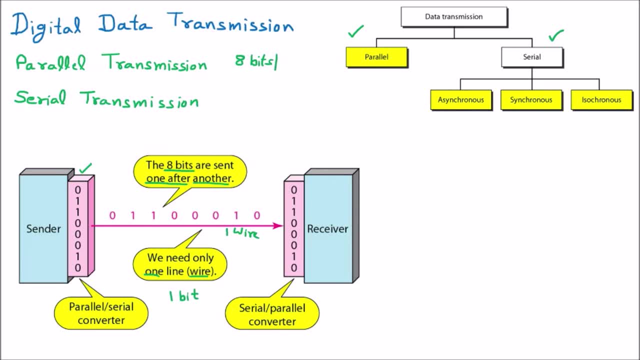 eight bits are sent per second, then here only one bit will be sent in a second. so this is the example of the serial communication. but yes, we know that the speed is less, but still we are using it because of the cost. that's why the people are more interested towards the cost and we are using it. now take this: 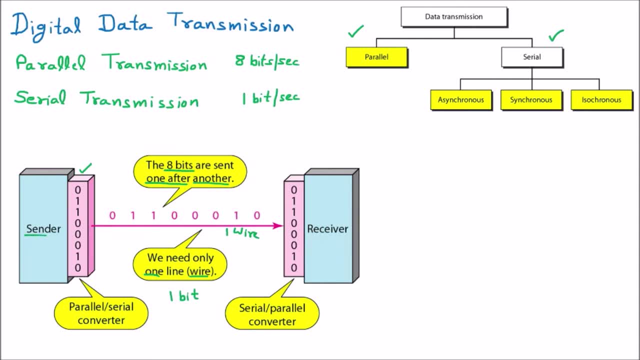 example, we are having a sender and we are having a receiver. so at the center side we are having some 8 bits and we have to send them. so only one wire is there through which those all 8 bits will come. and these are the parallel to 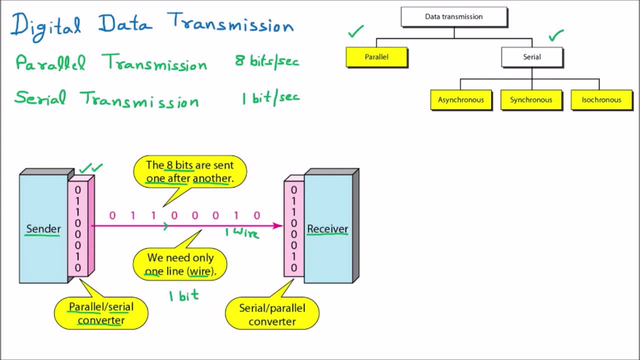 serial converter. this is applied. another side, again serial to parallel converter thing is that you assume that all the 8 bits are coming to the sender. means sender is sending the same 8 bits, but we are using only one line. that's why this converter is required. so this one is the converter which is converting the parallel to 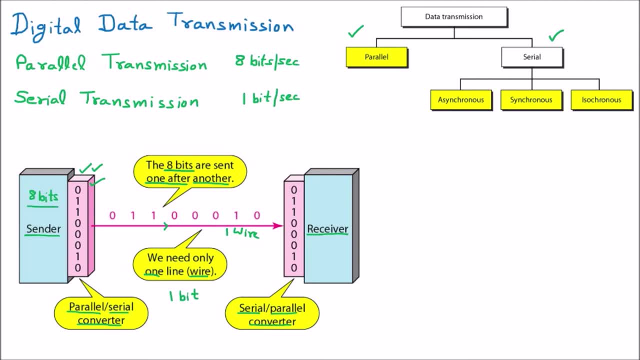 serial because these 8 bits are parallel and whatever they are going over, here they are, the serial. serial means 1, so converting 8 to 1, meaning I am giving them back to serial. and these are the 8 bits now coming here they are again. 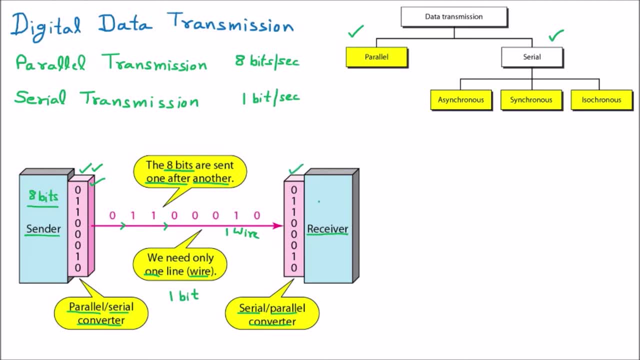 stored and again they are giving back. 8 bits are given here, so data was 8 bits only in both the cases, parallel and the serial. but the difference is that in the parallel 8 bits are sent in a second at the same time, because 8 lines are there. 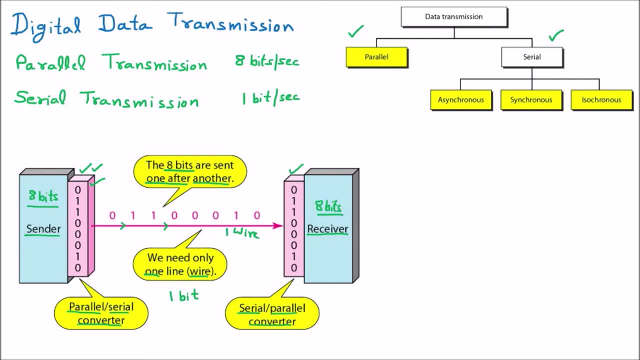 but in the serial we are having one line, so the 8 bit data is sent one by one, so after that another, so we can write about the serial transmission, that one bit sent with each clock tick, clock tick. we know that the clock will a second, am talking about 70 second. we can send only one bit, so that is the. 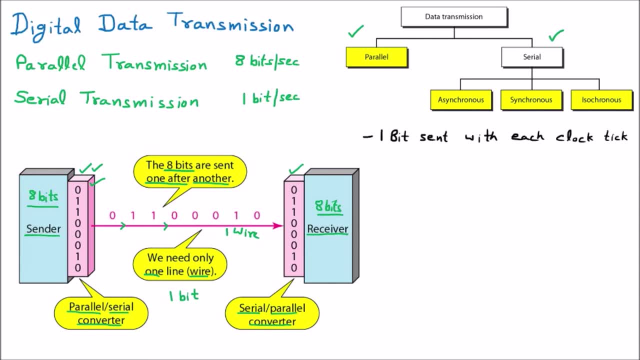 thing, only one bit is transferred and obviously, to transfer 1, this is going to 7. surely then is it moved to your reducer. if there is a yellow valid answer bit, we need only one line. so one line is required. so that is not a new thing we have to add on. 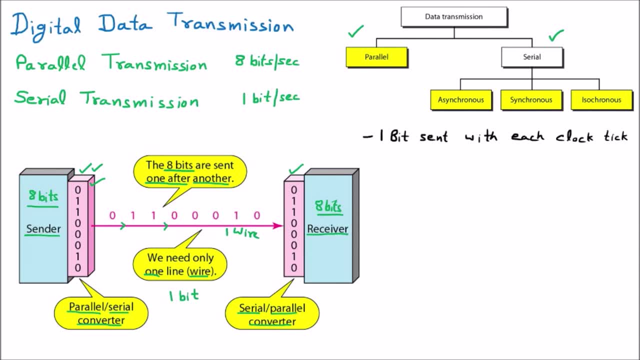 but yes, there are two important things in the concern with serial communication. one is the lsb- lsb stands for least significant bit- and there is another thing that is msp, which is called as most significant bit. now, least significant and most significant bit, now the right, most bit which is there, so bit at the right which is present, is the. 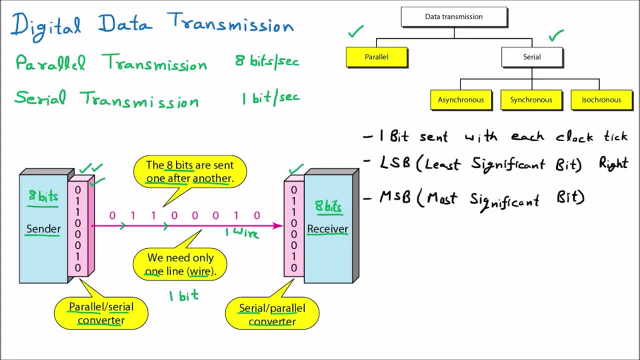 least significant bit and based on the left, that is called the most significant bit. so talking about here in the diagram. so here you can see that 0 is the on the right. so on the right we are having is the lsb least significant bit and here 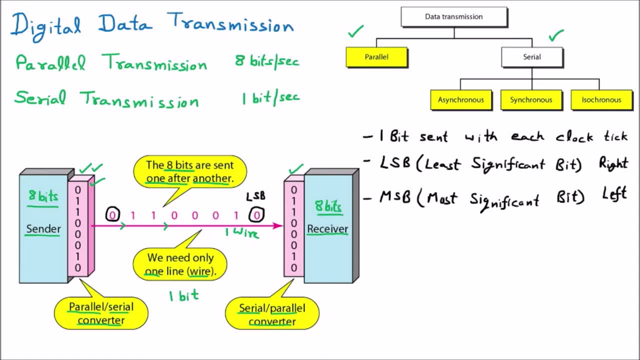 we are having 0 at the end, so that is the msp and the data is moving in this way. so which one is? the first bit transferred lsb, so we can write here: the data is transferred from lsb to lsb to msb. so, talking about the data, if we are sending the least significant bit will reach to the 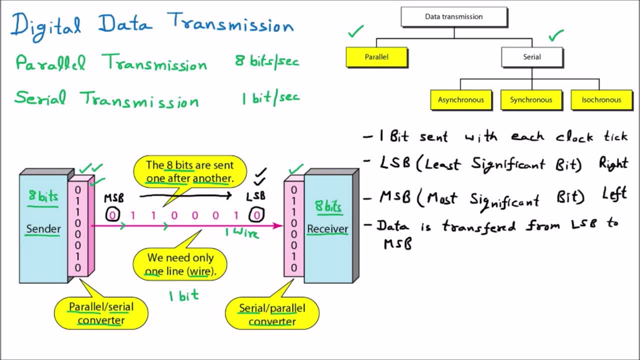 receiver first. so this is the bit which will receive to the receiver first, then afterward the chance is given. so on till the msp. so this is all about the serial communication. now we are talking about the advantages. so the advantages of the serial communication, the first and the foremost advantage. we know that it is the serial communication which is the 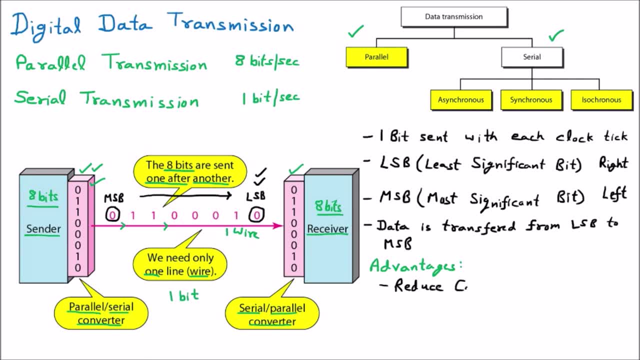 is the reduced cost. the cost of data transmission is very less because you know that only one line is going instead of eight lines. all the speed is less, no problem. but cost is very less and you know that today people prefer cost right. so less cost is there and that is also beneficial for the 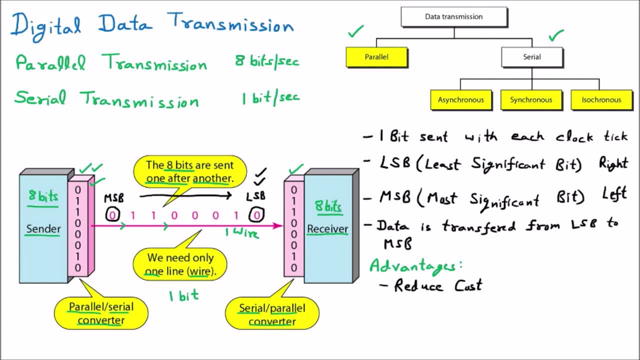 long distance. so that is much beneficial. now we are talking about the disadvantages, so disadvantages, so talking about the disadvantage, we need, or we require conversion device. well, we know this thing. here these two devices are extra. one is parallel to serial communication and then in serial to parallel, so that converter are required, because 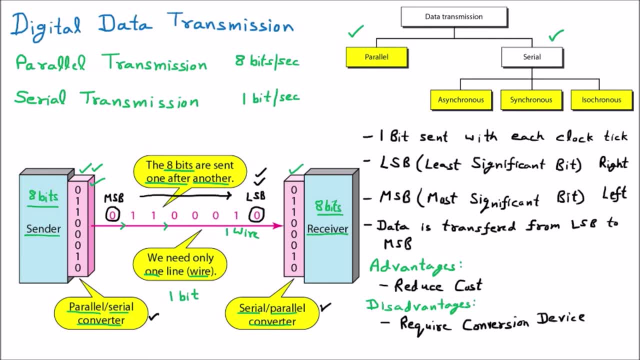 the sender is sending the data into the eight bits, then afterward those bits are converted to you, the serial communication, so that parallel to serial converter is required. then this serial reads to receiver and again the serial to parallel is converted, then given the eight bits to the receiver. so these conversion devices are required. so these are the extra, now afterward the serial.